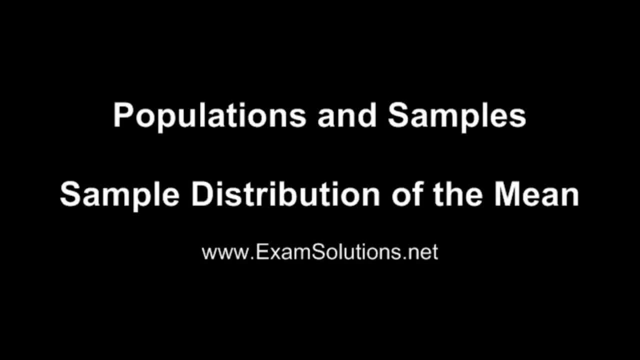 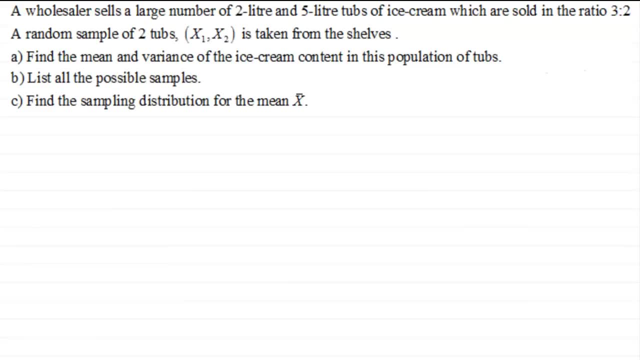 Hi, welcome to this video where we're going to look at the sampling distribution for the mean x-bar And to do this I've got a question here, which is fairly typical of the type of questions that you're likely to get on this. 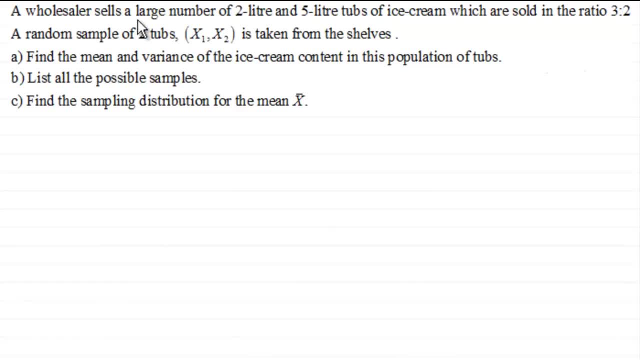 We've got a wholesaler sells a large number of 2-litre and 5-litre tubs of ice cream which are sold in the ratio 3 to 2. And a random sample of two tubs- let's say x1 and x2, is taken from the shelves. 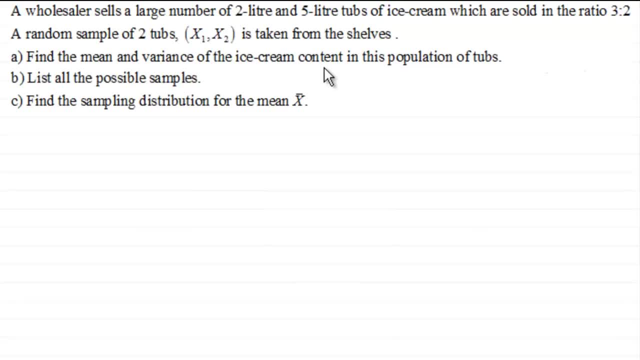 And in part A we've got to find the mean and the variance of the ice cream content in this population of tubs, And in part B list all the possible samples. And then finally, in part C we've got to work out the sampling distribution for the mean x-bar. 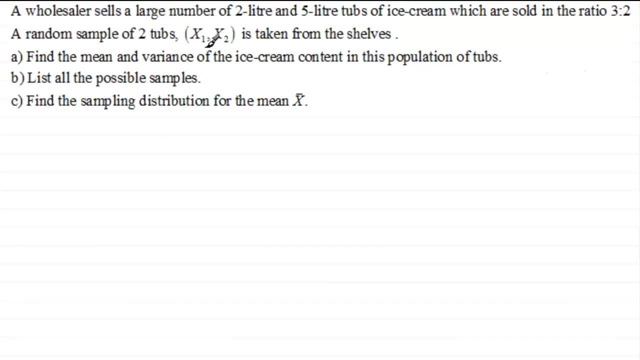 Now for the first part of the question, where we've got to find the mean and variance of the ice cream content in this population of tubs. what we need to do is set up a probability distribution table for the population. So if I was to say, let x be. 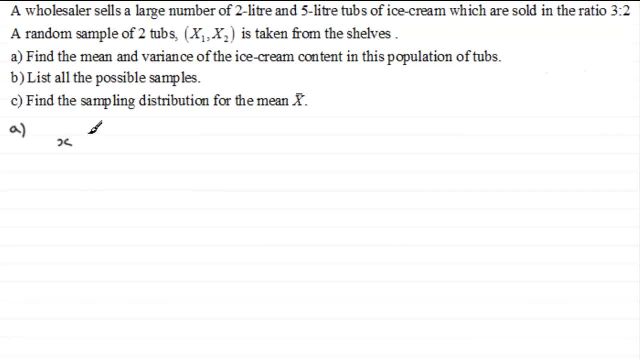 the type of ice cream that's sold, then the observed values are going to be a 2-litre or a 5-litre tub of ice cream, And so we could work out those probabilities, the probability of selling, say, a 2-litre tub. 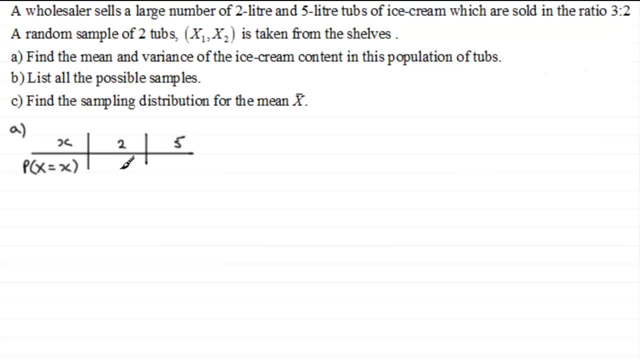 Well, it's going to be 3 out of 5, three-fifths, So that probability there is three-fifths. And then for selling a 5-litre tub, it's going to be 2 out of 5, two-fifths. 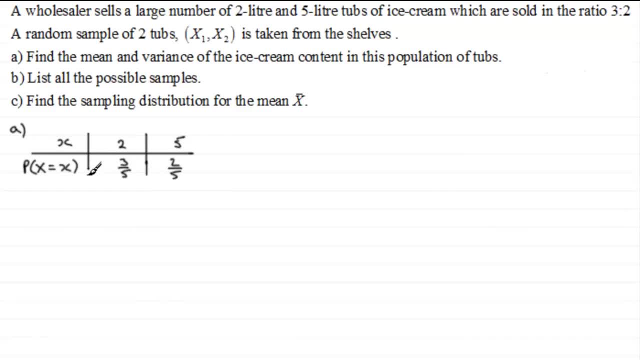 So we've got our probabilities here, then, And now we can go on to work out what the mean mu is. OK, we'll define it then as the population mean mu, And to work this out from a table like this, we should be familiar with this result from earlier work. 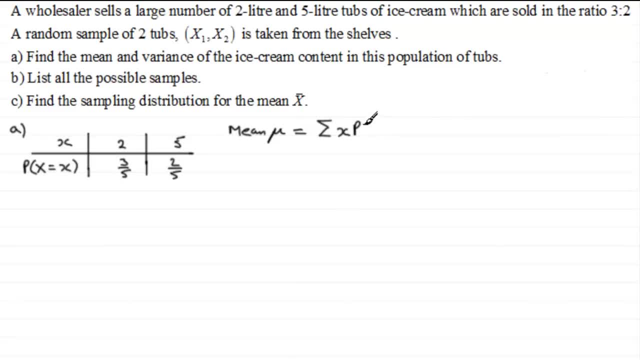 It's sigma: the sum of the observed value times the probability of getting that observed value, And if we carry that out for this table, we've got then 2 multiplied by three-fifths, And to this we add 5 multiplied by two-fifths. 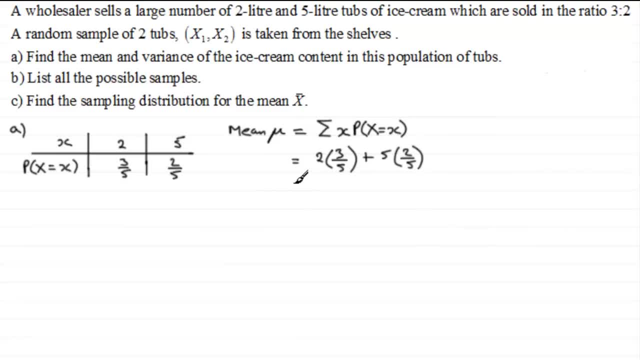 And if you work this out, you've got six-fifths plus ten-fifths, which is a total of 16-fifths, Or, as a decimal it's going to be 3.2.. And the units will be litres. 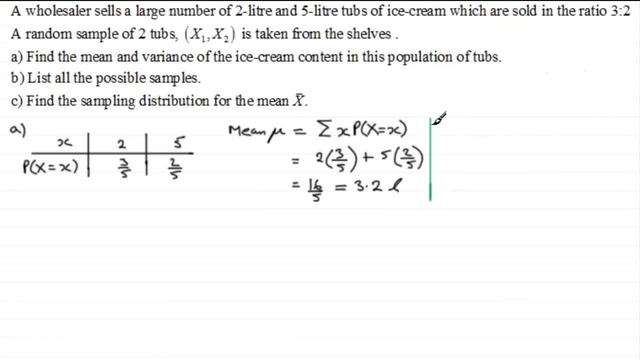 Now for the variance. let's just put that as VAR for short. The variance, which we'll say is sigma squared- OK, is equal to the sum of- and again, we should be familiar with this formula- the sum of the observed value squared multiplied by the probability of getting that. 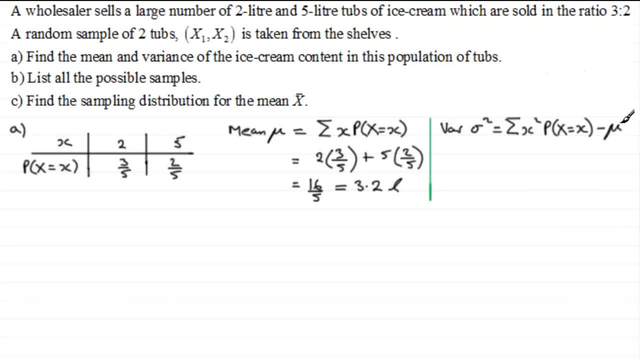 observed value minus the mean squared. So for this it's going to equal the observed value, two squared times three-fifths, two squared, then times three-fifths plus, and then the next observation was 5, so we've got 5 squared multiplied by two-fifths, and then from this we subtract 16-fifths. 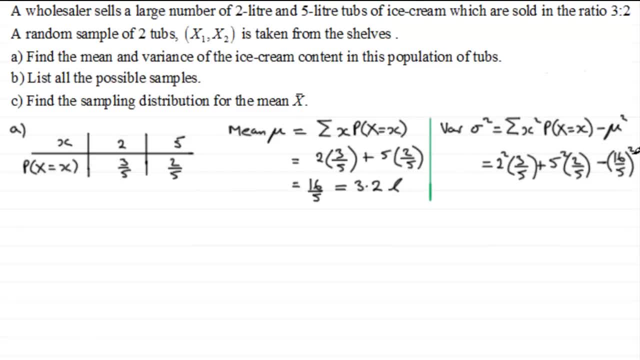 all squared, OK, the mean squared, And if you work this out, you will find you get 54, twenty-fifths, Or, as a decimal, that's 2.16.. And the units will be litres squared. OK, so we've got our mean and variance for the ice cream content, then of the population. 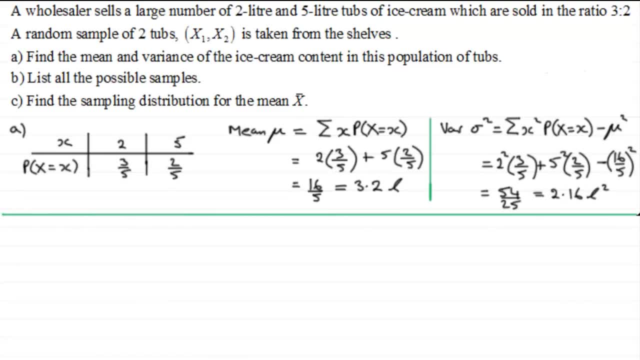 So we move on to the next part now, which is to list all the possible samples of size two that we take from the shells. So for those samples in part B, let's just put samples down here. What can we have of size two? 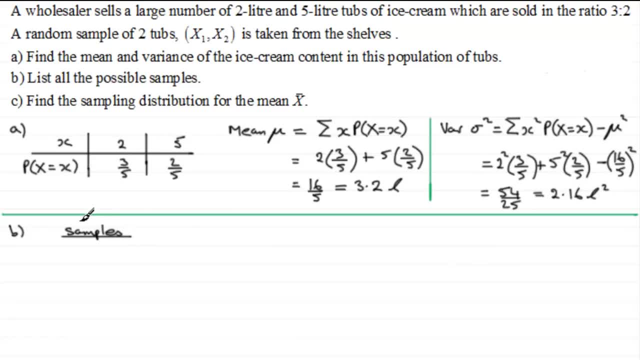 Well, we could pick two two-litre tubs of ice cream, So we could have a two-litre tub, One, two-litre one and then another two-litre one. What else could we have? Well, we could have say, a two-litre followed by a five-litre. 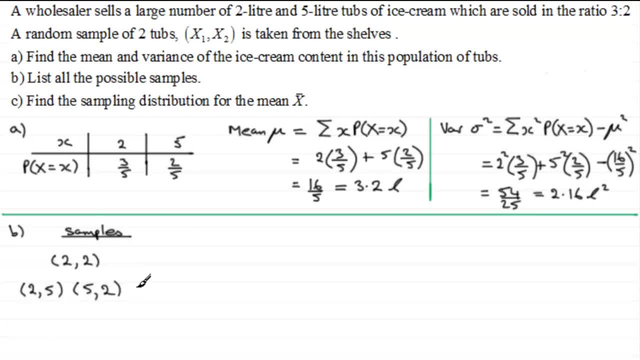 Or a five-litre tub followed by a two-litre tub, And finally you could get two five-litre tubs, And it's a good idea just to check in situations like this, that you've covered all the samples, And it's very easy to do. 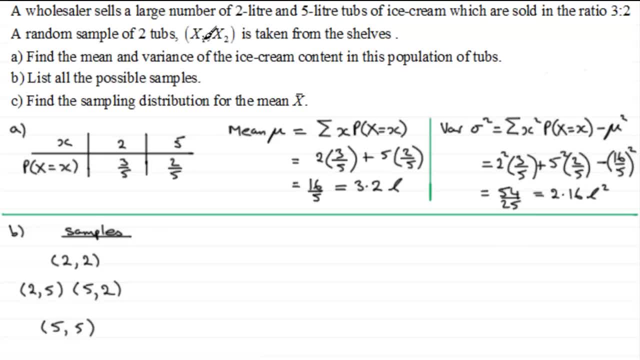 Because we could choose the first tub in any of two ways. We could have a two-litre or a five-litre there, And we could choose the second tub in any of two ways: A two-litre or a five-litre tub. 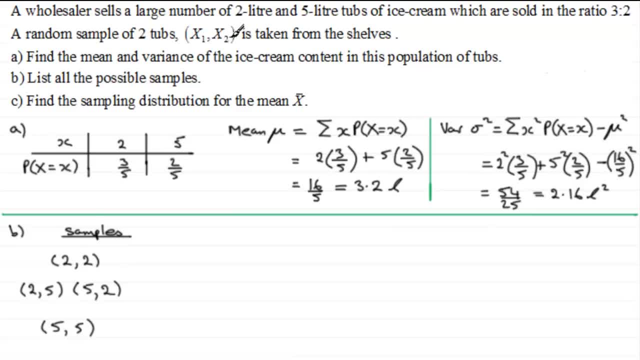 So it would be a total of two times two, A total of four samples that we can take. So it's a good check to do. OK, so, moving on from here, let's just section this off. We've listed all the possible samples. 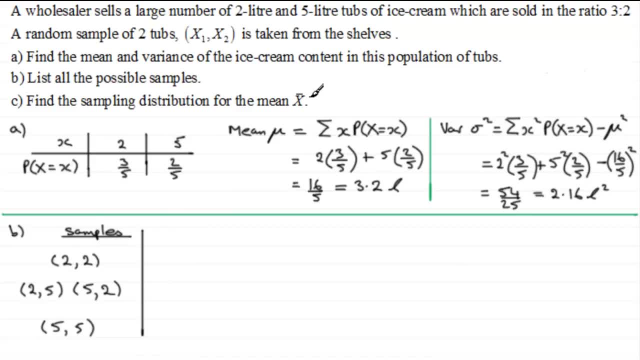 Now we've got to work towards finding the sampling distribution for the mean x-bar. Well, I need to work out what the mean of each of these samples is going to be, And for the first sample here, two and a two, the mean is going to be two. 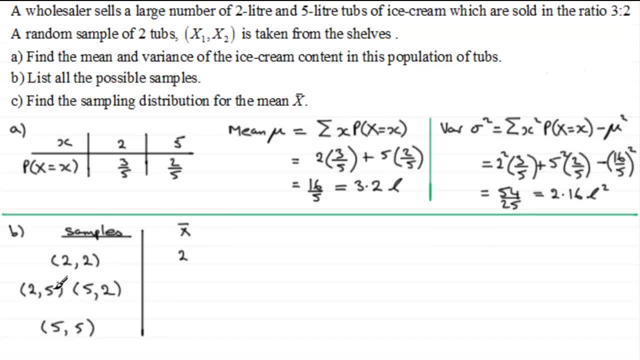 And for each of these two samples. if we add these two together, two and five is seven, divided by two is 3.5.. So the mean for each of these two samples is 3.5.. So the mean for each of these two samples is 3.5. 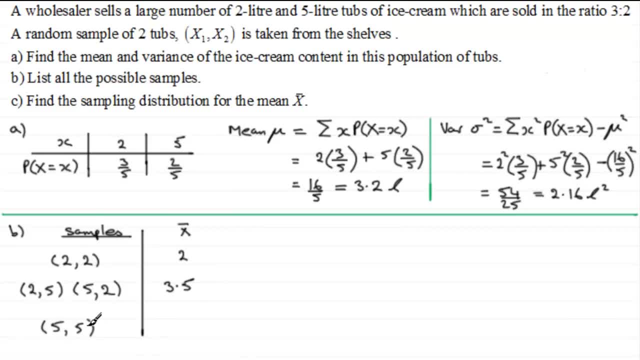 So the mean for each of these two samples is 3.5.. And lastly, for this five and a five, the mean is going to be five there. Now, when it comes to working out this sampling distribution, we now need to work out the probabilities of getting these various means. 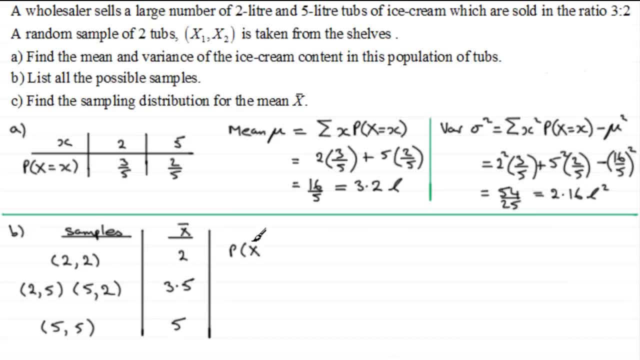 So the probability that the sample mean is equal to two is going to be. well, we would have a tub containing two liters, followed by another tub containing two liters. So that's going to be 3.5 multiplied by 3.5, or 3.5 squared. 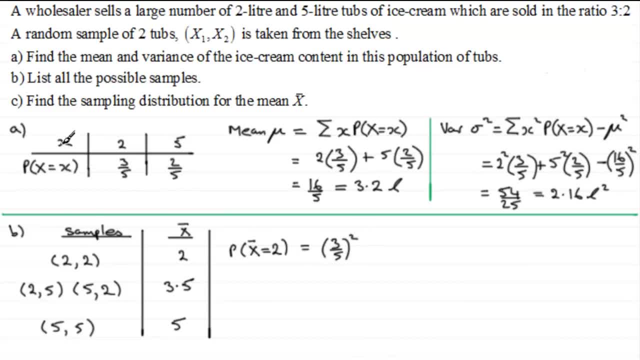 So that's why we needed our probability distribution for the population for this part of the question. Anyway, if you work this out, you end up with 9 over 25.. 9 twenty-fifths, And we carry on and we work out. now the probability that the sample mean is 3.5.. 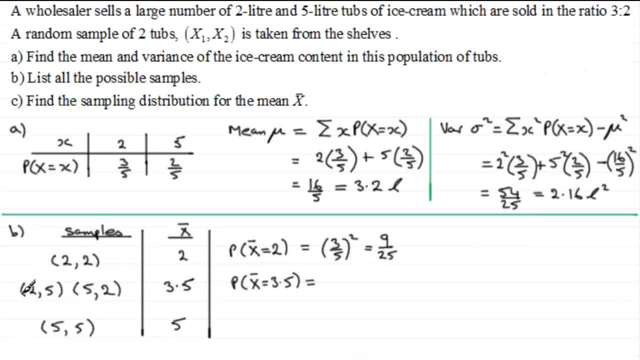 And for this one. well, if we were to work out for this sample the probability of getting it, it would be for a two. it would be a probability of three-fifths, followed by getting a five-liter tub, two-fifths. 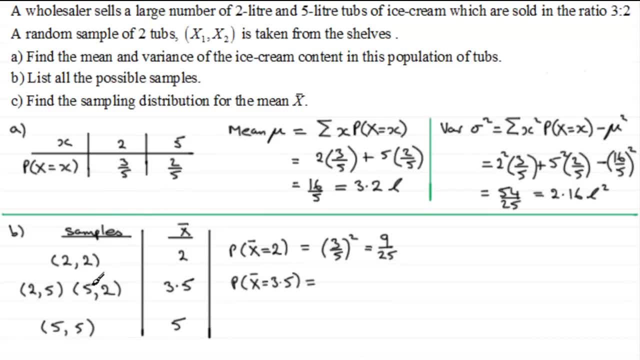 So it would be three-fifths times two-fifths. But you've got it again here. although it's the other way around, It's still going to be the same answer. So what we've got is two lots of three-fifths multiplied by two-fifths. 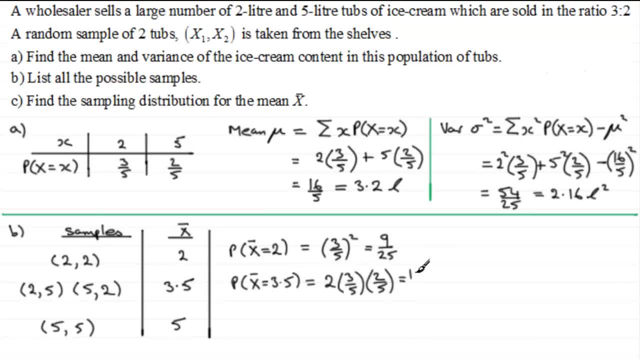 And if you work this one out, you'll find you get 12 twenty-fifths. Now for the last one. the probability of getting a sample- mean then of five- is just from this sample getting a five and another five. So it's going to be two-fifths times two-fifths. 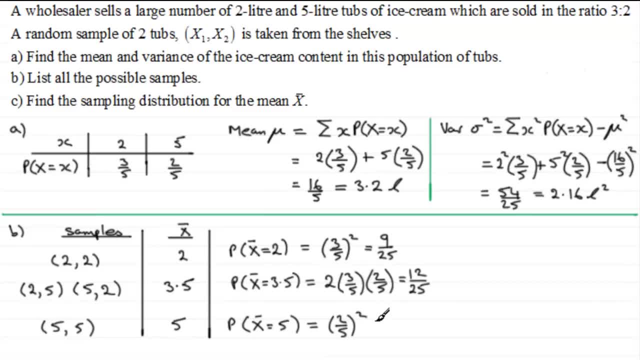 or two-fifths all squared, And if you work that one out, that is four twenty-fifths. So when it comes on to writing down what our probability distribution is for the sample mean x-bar, then let's just write a subtitle here that the distribution